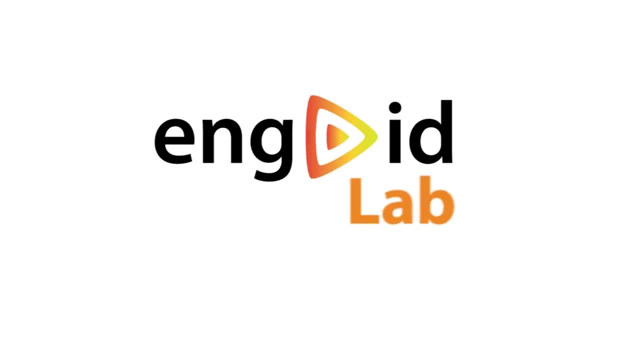 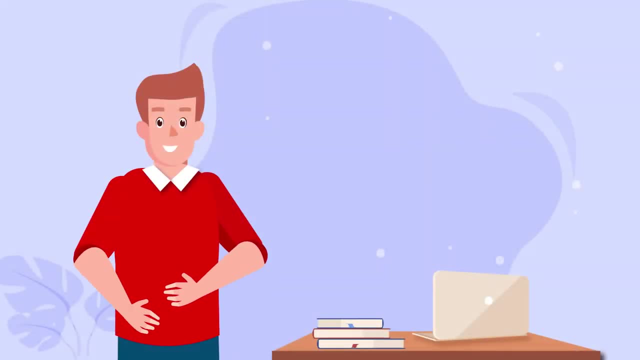 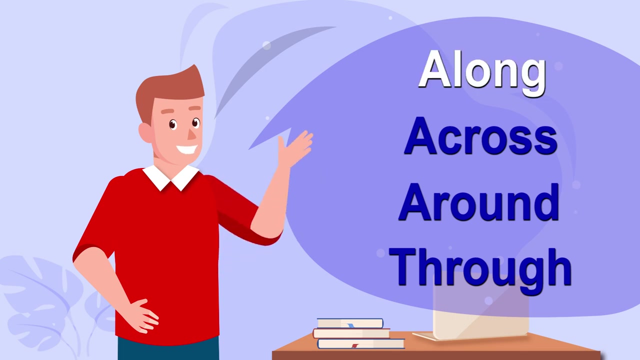 Hello everyone, Welcome back to EngVidLab. In this lesson, you're going to learn about four prepositions, and they are along, across, around and through. Okay, then let's get started. The words along, across, around and through are some of the prepositions of movement. 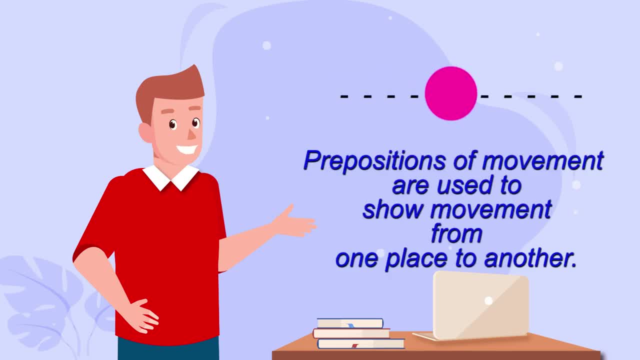 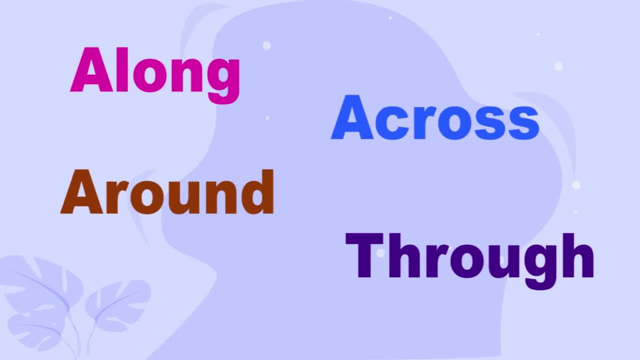 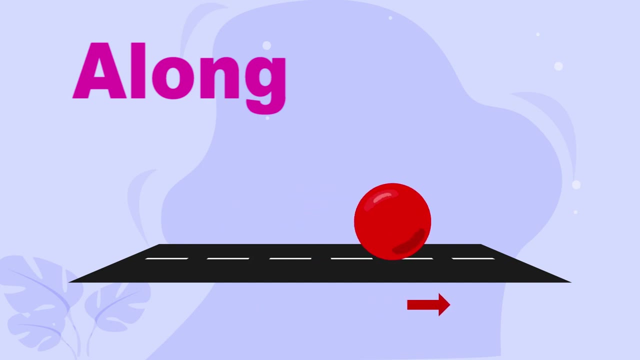 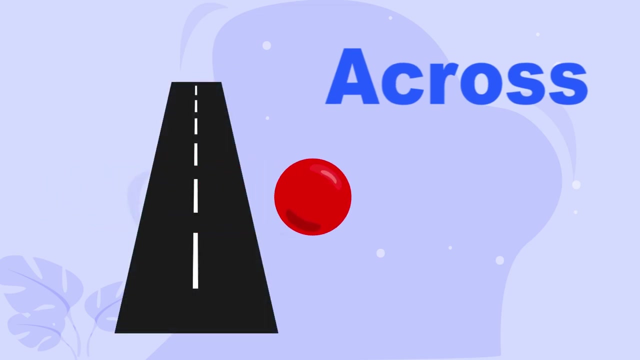 Prepositions of movement are used to show movement from one place to another. Let's look at the four prepositions one by one. We use the preposition along to show movement in a constant direction. We use the preposition across to show movement from one side to the other. 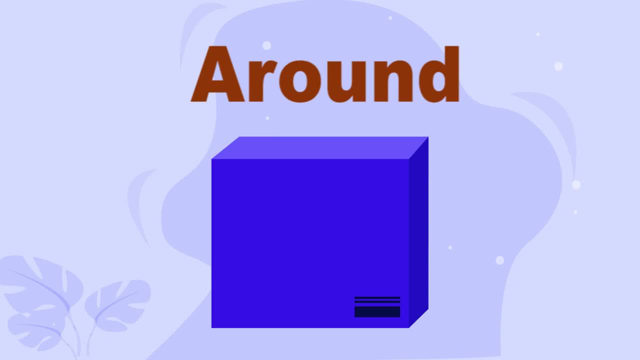 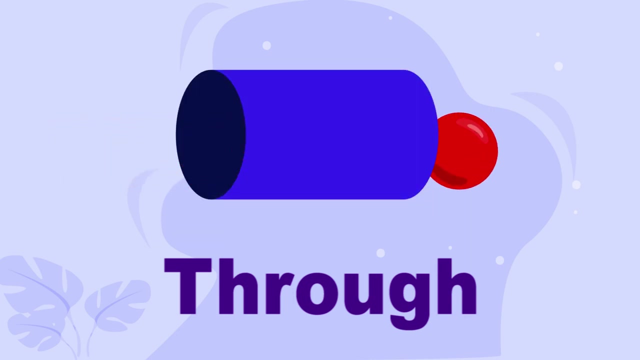 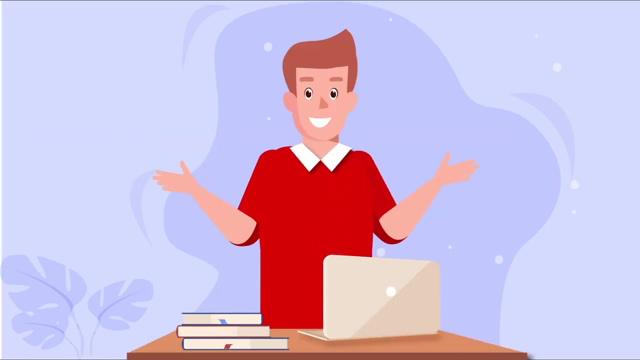 We use the preposition around to show movement on each side of something or direction surrounding something or somebody. We use the preposition through to show movement from one end of something to the other. Okay, then let's move on to the second part of the lesson, where I'm going to show you some examples for these words, using some images and animation. 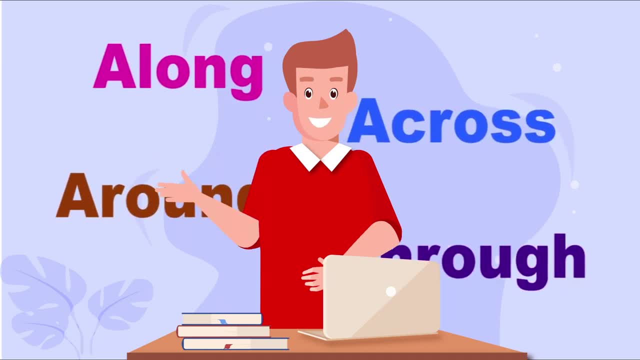 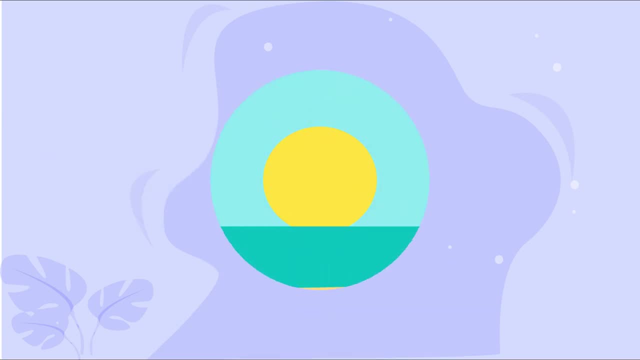 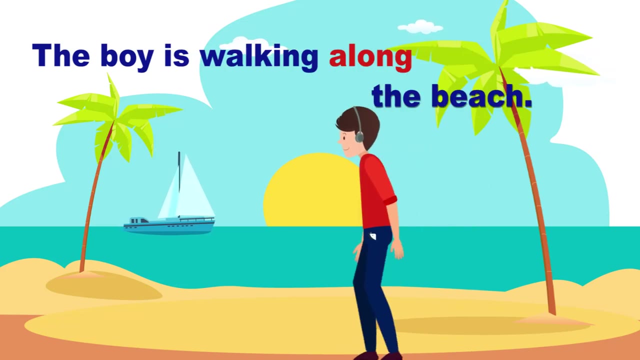 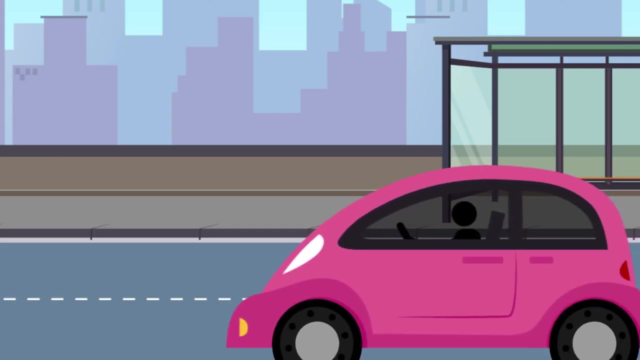 Okay, then let's move on to the second part of the lesson, where I'm going to show you some examples for these words, using some images and animation. The boy is walking along the beach. The boy is walking along the beach. The girl is riding a scooter along the road. 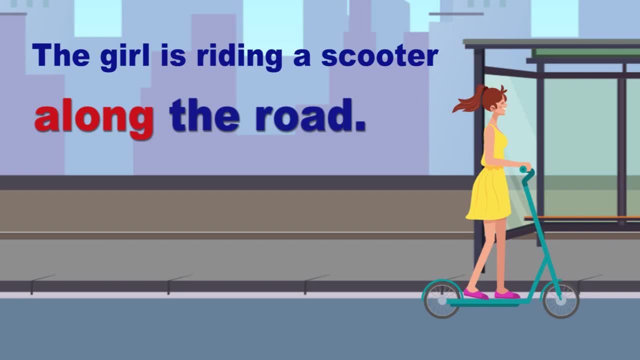 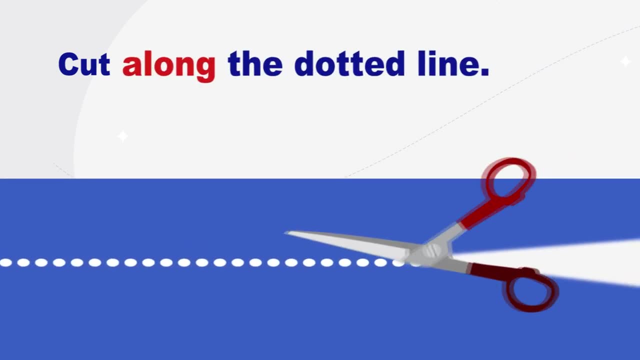 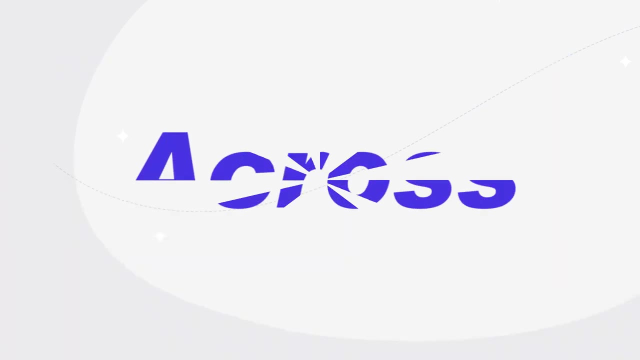 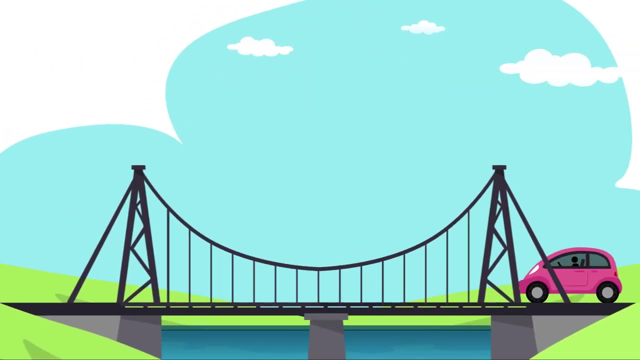 The girl is riding a scooter along the road. Cut along the dotted line. Cut along the dotted line. Cut along the dotted line. The car is going across the bridge. The car is going across the bridge. The car is going across the bridge. 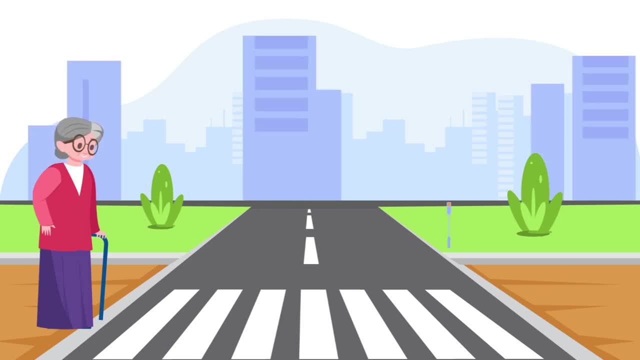 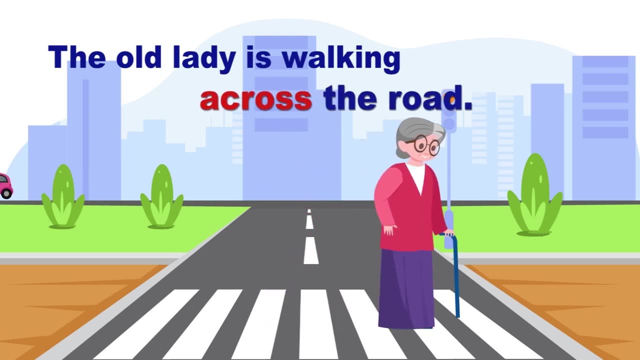